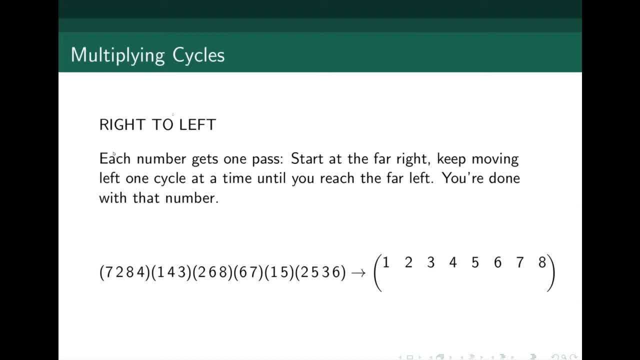 head while you're multiplying cycles is that it always goes right to left. We're going to start at the rightmost cycle and go one cycle at a time to the left until we reach the end. And how we're going to do this is one number at a time, So we're going to first. 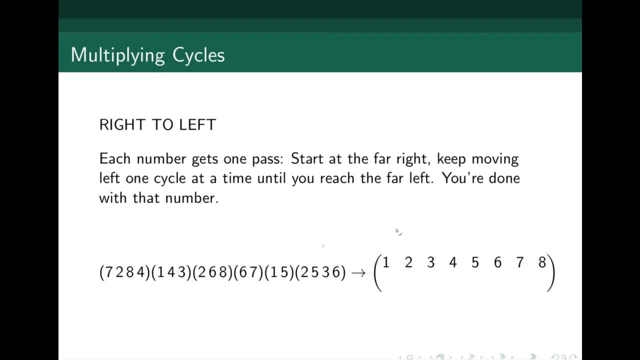 think about what happens to the number 1 from right to left, then what happens to the number 2 from right to left, And so the first thing I want to do is I want to start at 1.. I don't see a 1 in the first cycle. I do see a 1 in the second. 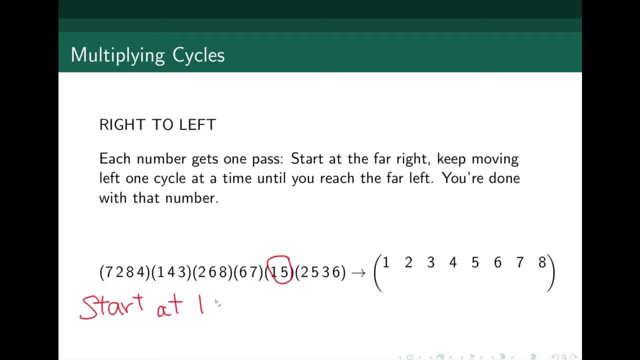 cycle, And in that cycle 1 goes to 5.. So I've started at 1 and I go to 5.. So now I'm at 5.. In the next cycle: nothing happens to that 5.. In the next cycle: nothing happens. 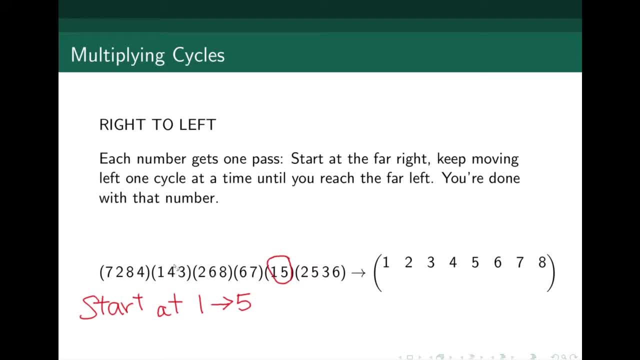 to that 5.. In the last cycle nothing happens to that 5. And now we're at the end. So we started at 1, we ended up at 5.. That means overall 1 goes to 5 in this permutation or this product. 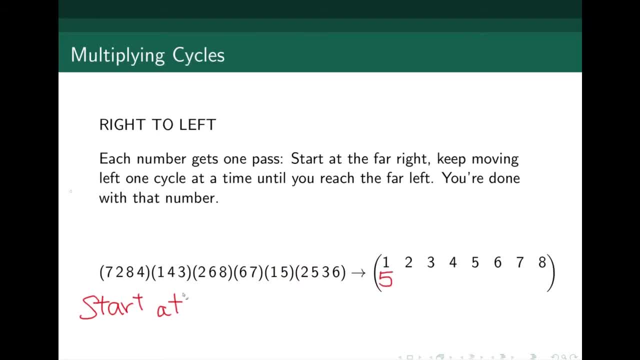 of permutations. if you want to think of it that way, Next time through we want to consider what happens to the number 2.. So we're going to start at the number 2 and see what happens. Well, in this first cycle I do see a 2.. What happens to the 2?? It goes to: 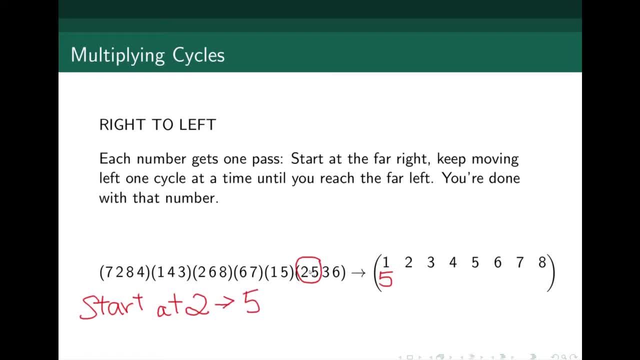 5.. So now I'm at 5.. In the next cycle, what happens to that 5?? It goes back to 1.. So now we're at 1.. Nothing happens to 1 in the next cycle. Nothing happens to 1 in the next cycle. In the next. 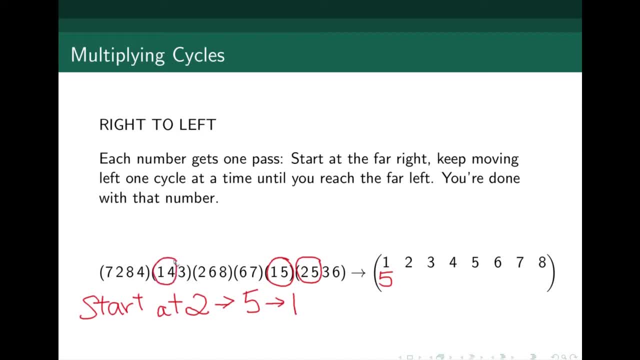 cycle we see that 1 goes to 4.. So now we're at 4.. And in the very last cycle we see that 4 goes back to the beginning, which is 7.. Now we're out of cycles, So we're completely finished with processing the 2. The 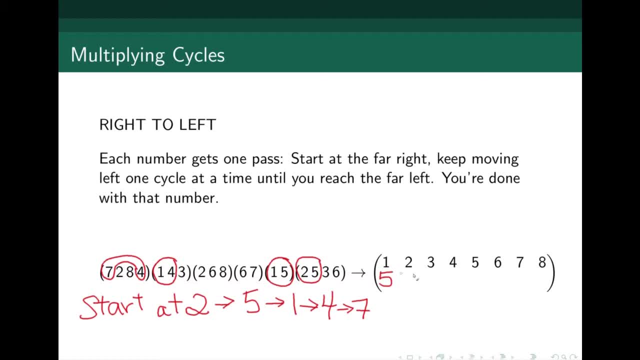 2 ends up at 7.. So 1 goes to 5,, 2 goes to 7.. Next we'll consider what happens to the 3.. If you're starting to feel comfortable with the process, I recommend you pause the video, figure out what happens to the 3, and then 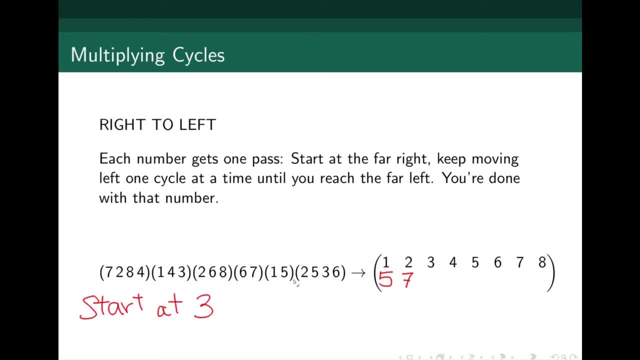 press play when you're ready to check your answer. But first we see that the 3 goes to 6, then nothing happens to the 6,, then the 6 goes to 7,, nothing happens to the 7, nothing happens to the 7, and finally the 7 goes to 2.. So we started at 3, we ended up at 2, so 3 goes. 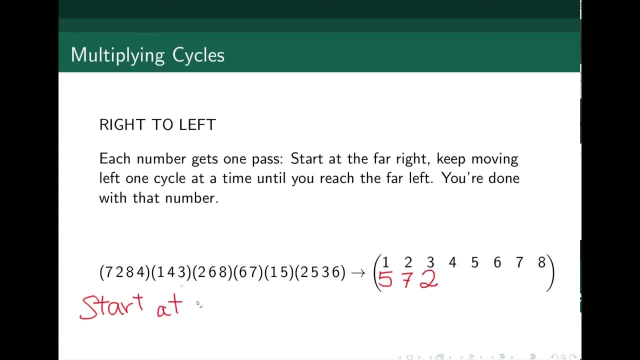 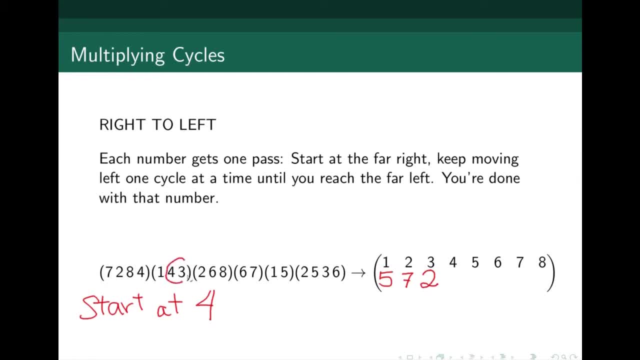 4. here, finally we find a 4, and it goes to 3, and then nothing happens to the 3.. So 4 ends up at 3.. Next let's consider the 5.. First it goes to 3,. nothing happens to 3 here. 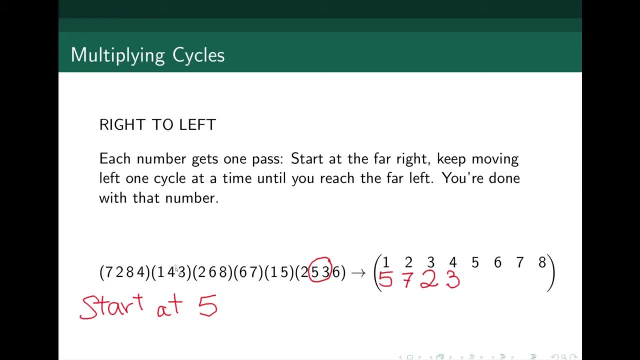 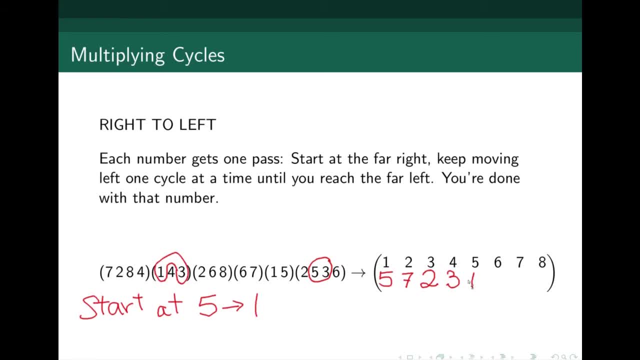 ends up at 1.. Now let's look at 6.. 6 first goes to 2, nothing happens to 2, nothing happens. nothing happens to two. two goes to six. nothing happens to six, nothing happens to six. So the six ends up at six. 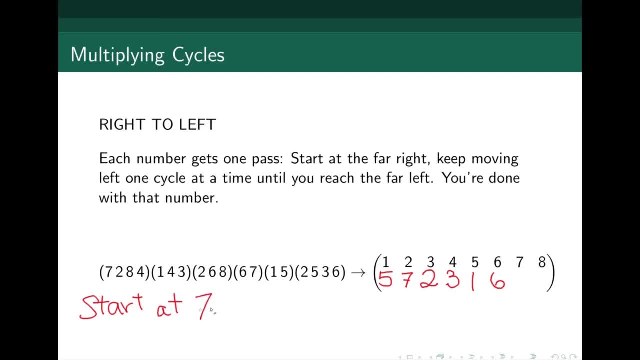 Next we consider what happens to the seven. so we'll start at seven. nothing happens to seven here. nothing happens to seven here. seven goes to six. here six goes to eight. nothing happens to eight, and then eight goes to four. 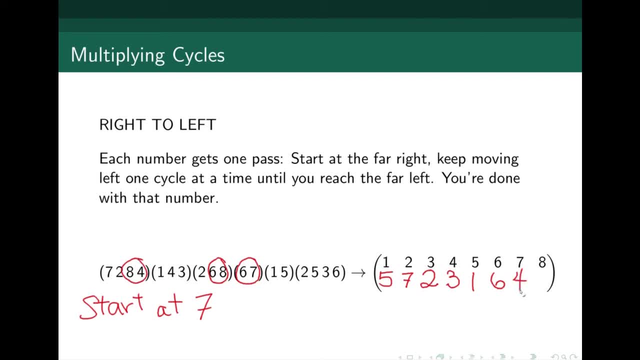 So the seven ends up at four. Finally, we're ready to talk about the eight. What happens to eight? Well, nothing happens to eight in the first cycle, nothing happens to eight in the second cycle, nothing happens to eight in the third cycle. 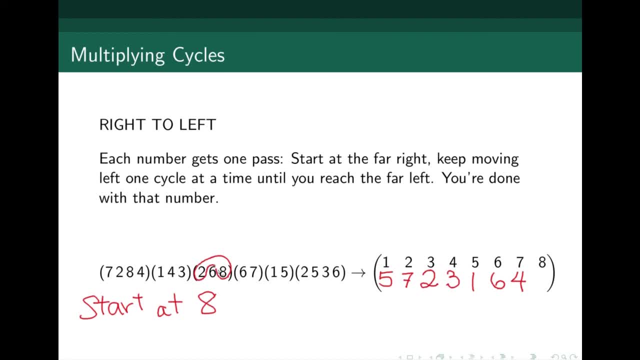 Here we find an eight that goes to two, nothing happens to two, and then two goes back to eight. So at the very end eight ends up at eight. So when there are repeat numbers in our product of cycles, we have to make sure we process from root to root. 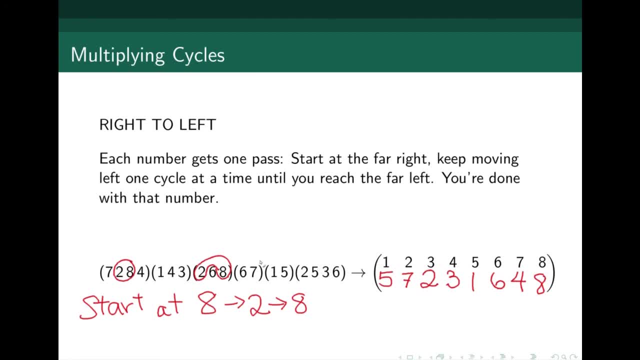 We have to make sure we process from root to root. We have to make sure we process from root to root, right to left, not from left to right or in random order. It must go from right to left, one cycle at a time. Figure out where each number ends up. So finally, in two row notation, the bottom row reads: 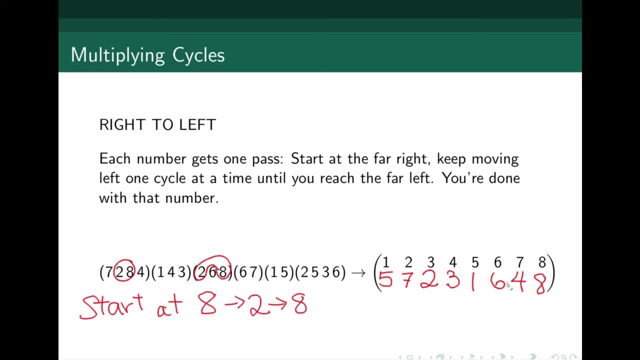 5,, 7,, 2,, 3,, 1,, 6,, 4, 8 for this product of overlapping cycles. In the quiz for today, you'll get some practice with these multiplications and also with some of the conversions from the first.